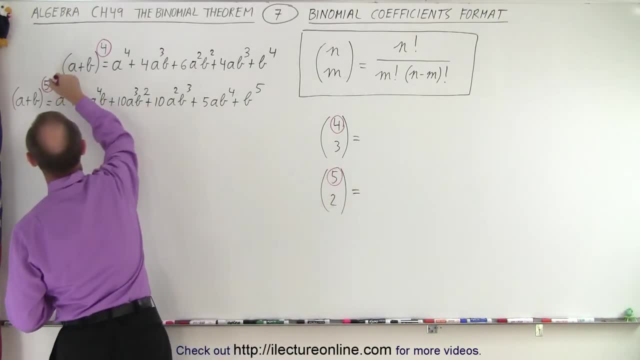 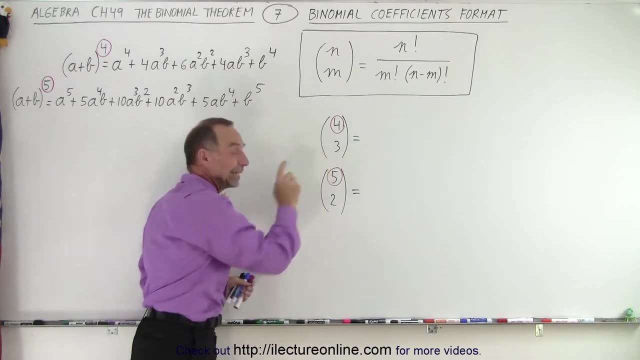 number five is equal to the number five over here. So the top number indicates the exponent of the binomial expansion. The bottom number indicates the exponent of the second term in the binomial expansion. So here you see three, and we're looking for the term that. 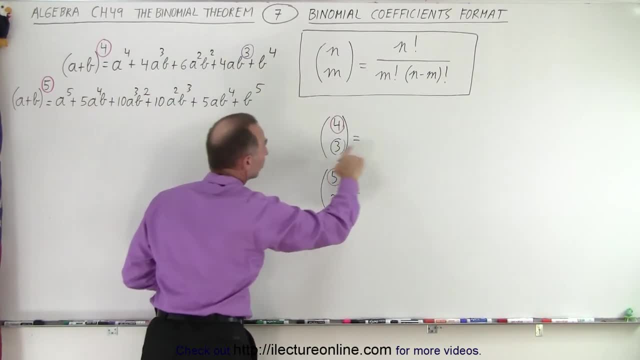 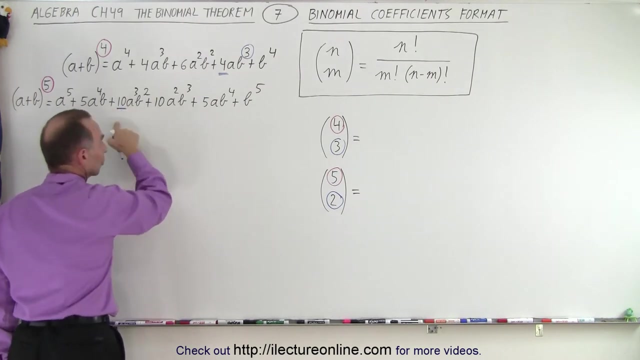 contains b to the third power, which is this: The result of this calculation will equal the numerical coefficient of that particular term. In this example, here we're looking for b to the second power, which is right here, and so we're looking for this numerical coefficient. 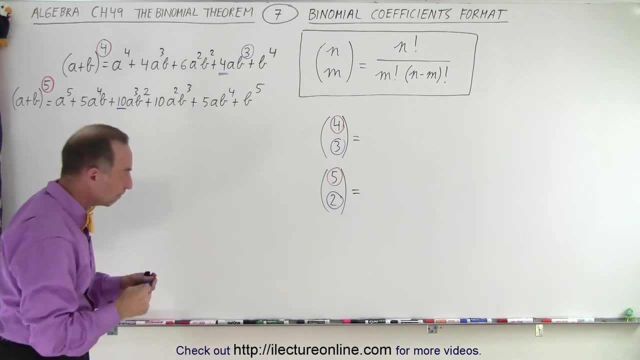 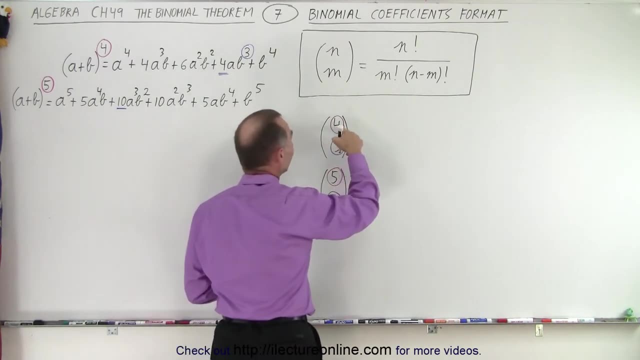 which we will get when we expand this out the way it's written. Let's go ahead and work this out and see what that looks like. So here on the top we have four factorial Four. that's the top number. So we have four times three. 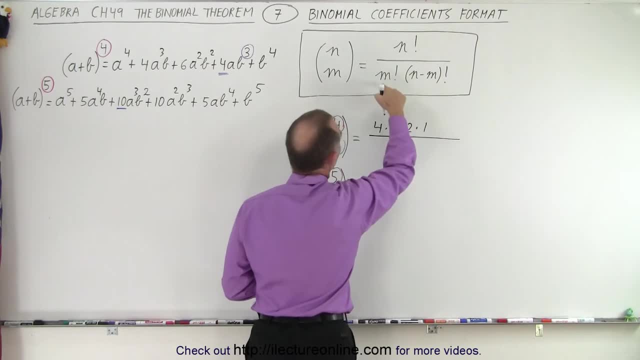 times two times one, divided by m factorial, which in this case is three. Three times two times one, multiplied times n minus m factorial, So this would be three. no, that would be four, not three, but four minus three factorial. So you can see that's four factorial divided by three factorial times the difference between the two. 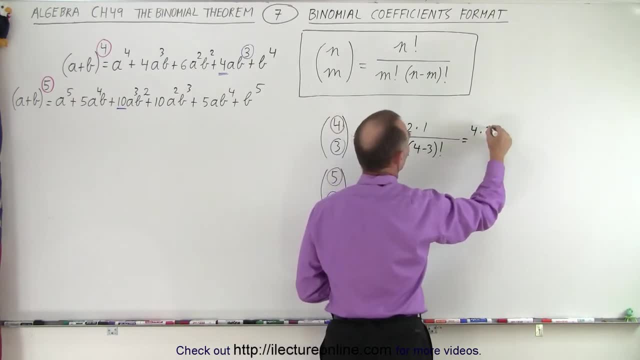 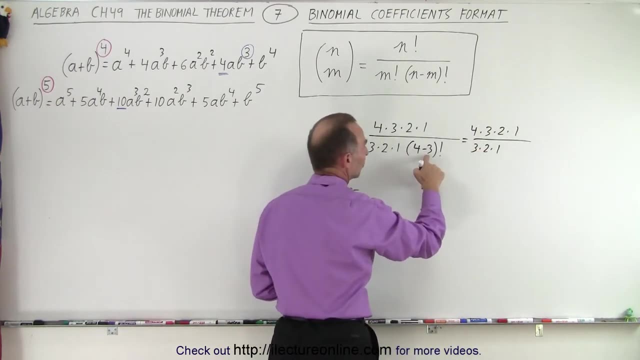 four minus three factorial. So this becomes four times three times two times one, divided by three times two times one, and of course, four minus three, that's one factorial. And if you remember, one factorial was equal to one, so times one. Now you can see that you can. 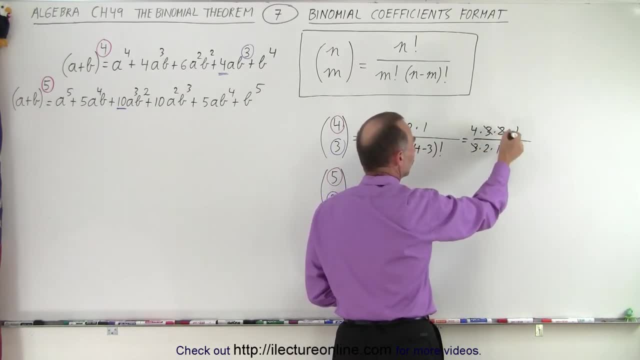 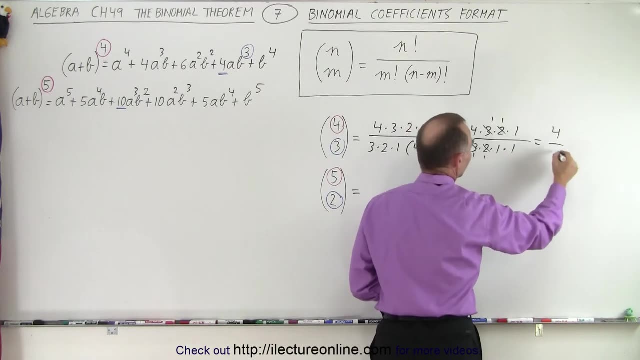 easily simplify this. You have a three in the numerator and the denominator. You have a two in the numerator and the denominator, So this becomes one and one, And so this becomes in the numerator. four divided by the denominator is one and simply equal to four. 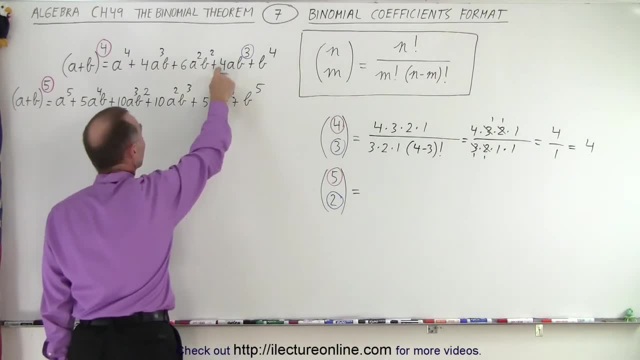 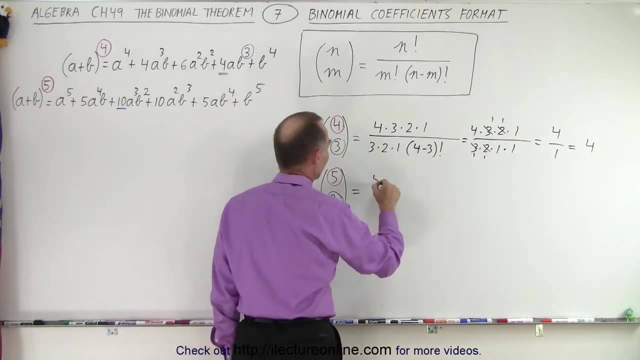 And notice, that's the number we were expecting, because that's a numerical coefficient of this particular term. Let's see if the second one works out that way as well. So here we have five factorial divided by two factorial times five minus two factorial. So we'll go ahead. 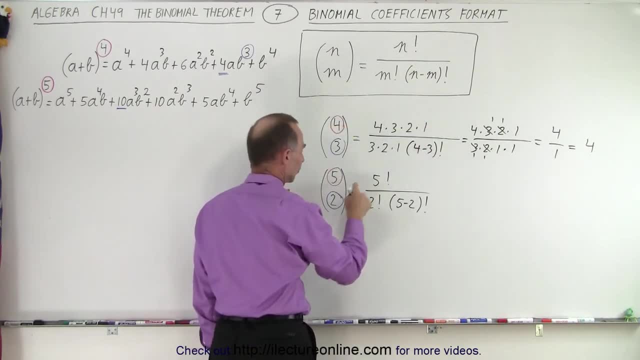 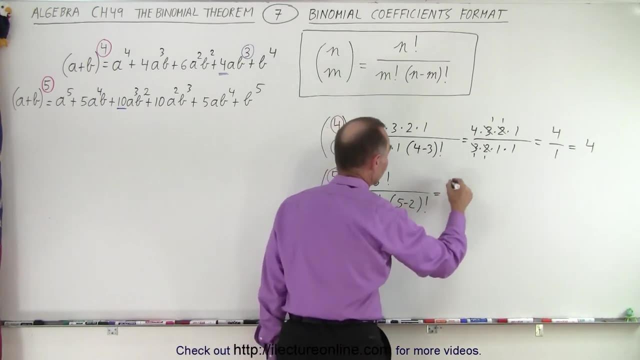 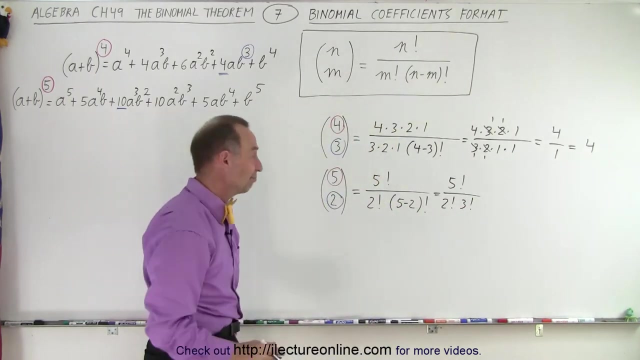 and write it out exactly the way we have it there. So the top number five factorial, the bottom number, two factorial, And then the difference between the two factorial. So that becomes: this is equal to five factorial divided by two factorial times three factorial. And now we can simply write it out. Now, often you 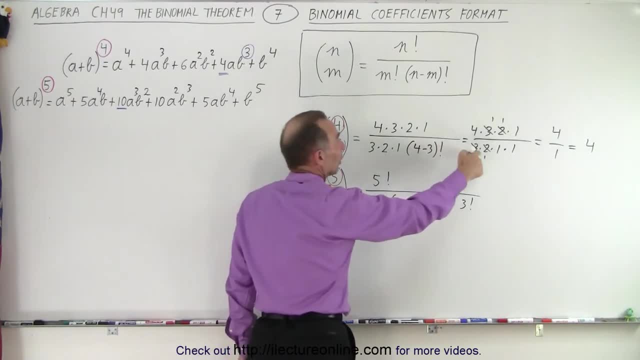 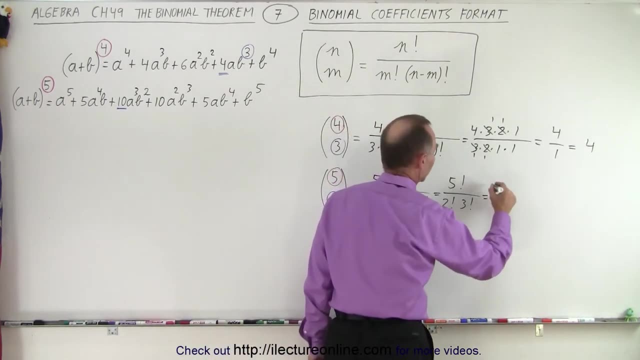 don't need to go to these steps. You can simply look at this and go directly to this format, if you like. So whatever you feel most comfortable with. Or you can simply go to the steps, one at the time. So this becomes five times, four times, three times, two times one divided by: 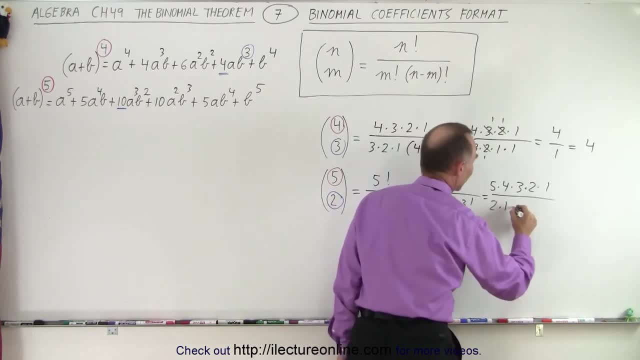 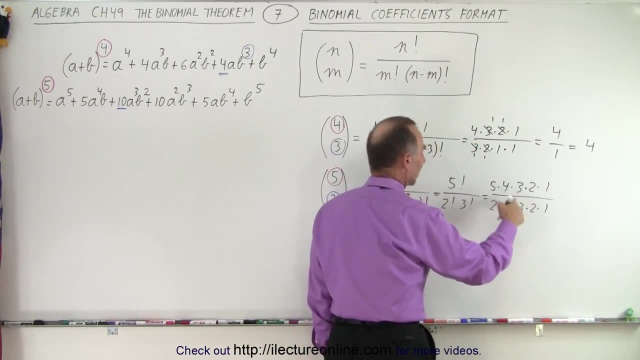 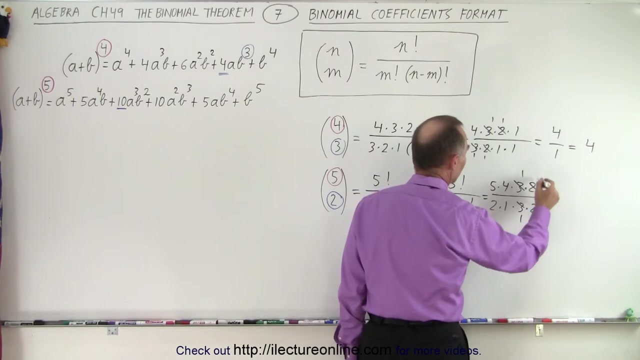 two times one for two factorial times, three times two times one, which is three factorial. So we have two factorial times, three factorial in the denominator and five factorial in the numerator. Now we can simplify that. Notice: the three cancels out with the three, the two cancels out with the. 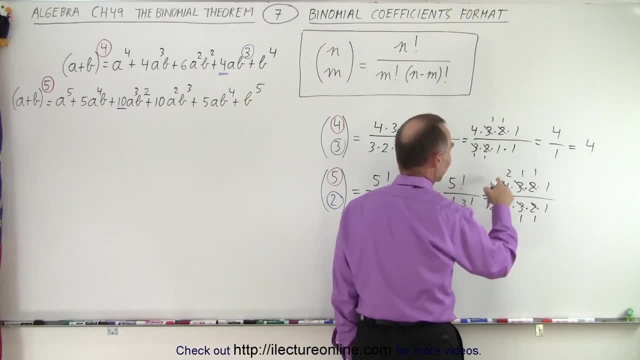 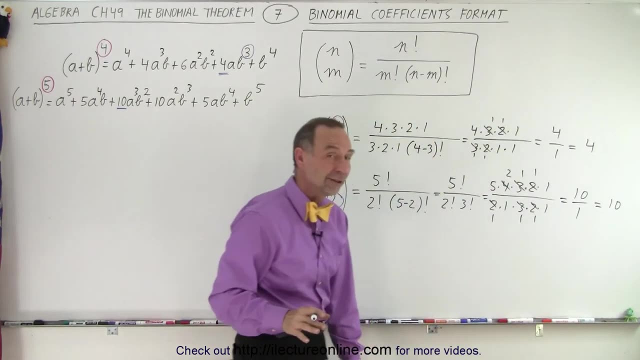 two and this two cancels out with that four. Now we have five times two, which is ten in the numerator divided by all ones in the denominator, which is equal to ten. And again, notice, we got the right answer. the answer: we're looking for the numerical coefficient of this term. 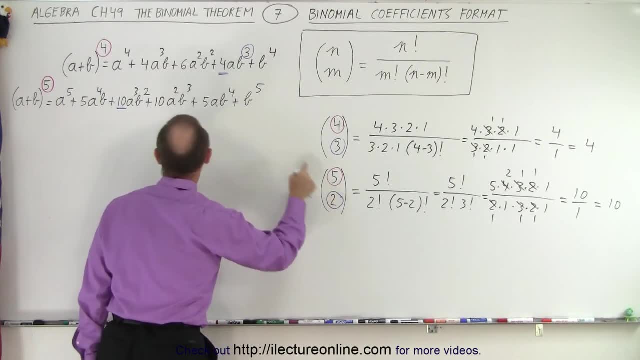 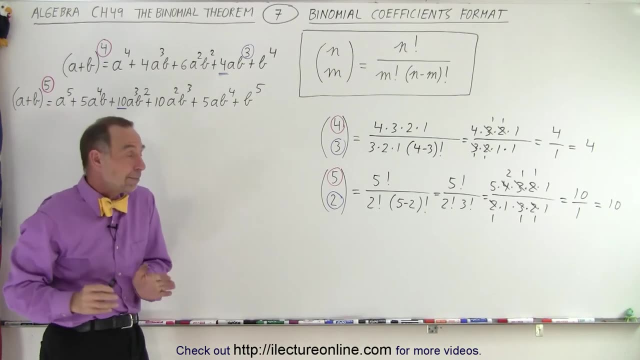 where b squared, that's the two right there, and five is the exponent of the binomial expansion. so you can see this is a very slick, quick method to find any numerical coefficient of any term in the binomial expansion, and it can be done quite quickly when you use numbers like this. 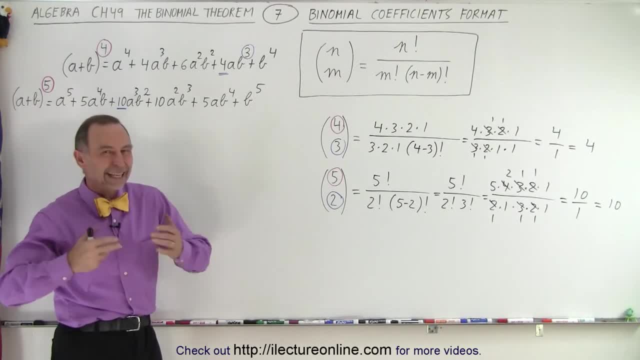 and examples like that. now, when the numbers get a little bit bigger, it takes a little bit more work to get to the arithmetic, but the method will be exactly the same and that is how it's done. so that's a good question: what's easier? to do this or to do pascal's triangle, and sometimes 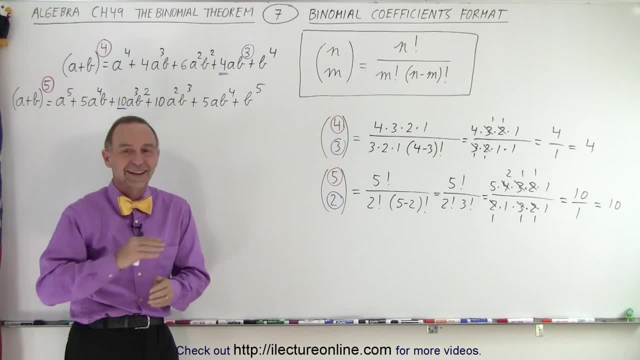 pascal's triangle, especially for the smaller exponents, is quicker than to go ahead and use this method. it's when you get up to some very big numbers that you probably want to go here rather than use pascal's triangle. can you give a big number to have all? 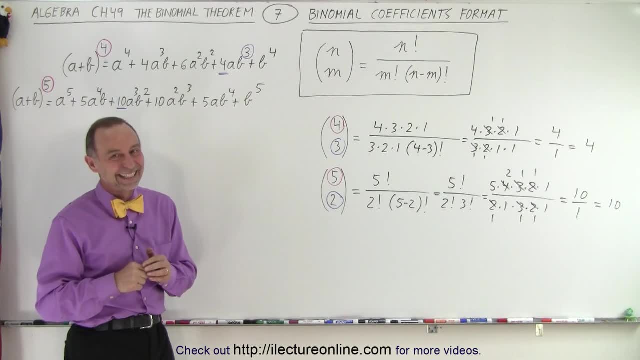 yes, it's when you have to get it for all of them. it becomes a lengthy process, but sometimes they only want the first or the third or the fourth one, and then it becomes a lot easier to do this. we'll show you some examples.